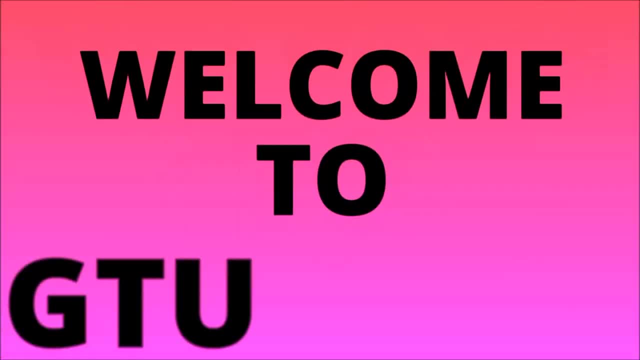 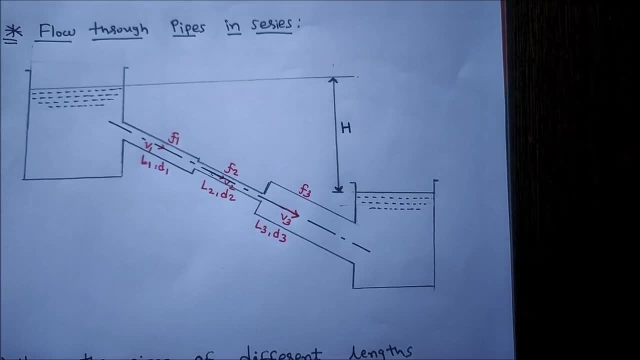 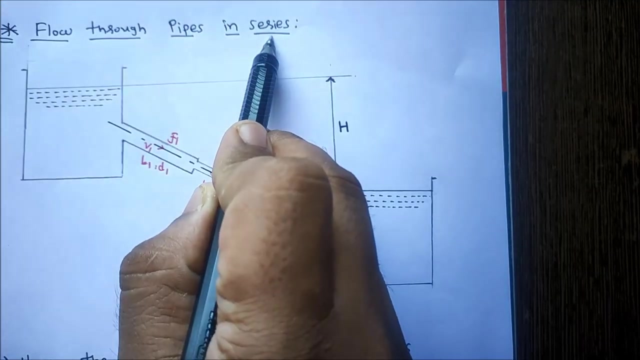 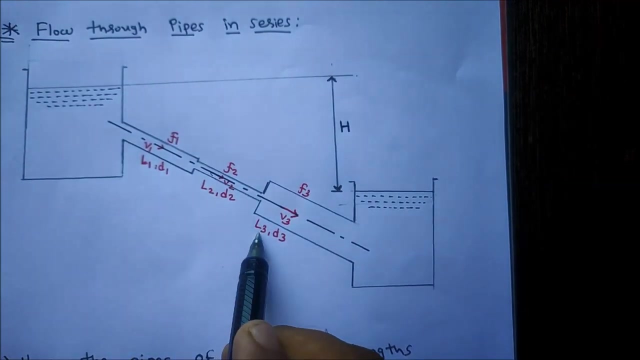 Hello friends, today we discuss about flow through pipes in series or flow through compound pipes. So first question is: what is the meaning of pipes in series? Here we take three pipes of different length and different diameters Here: L1, L2 and L3. that are the length of 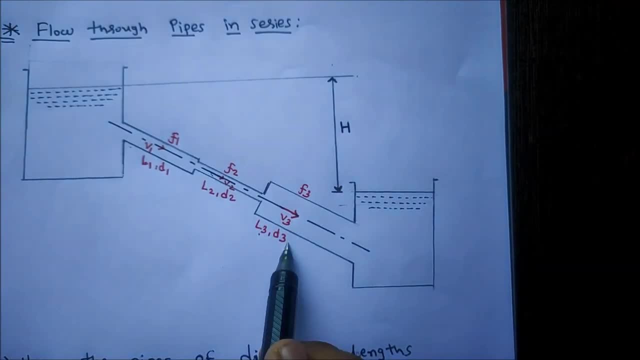 this pipe: 1, 2 and 3 and D1, D2, D3. that are the diameters of this pipe. So when the pipes of different length and different diameters are connected end to end to form a pipeline, then such a pipeline is called as a compound pipe or pipes in series. Again, I repeat: when 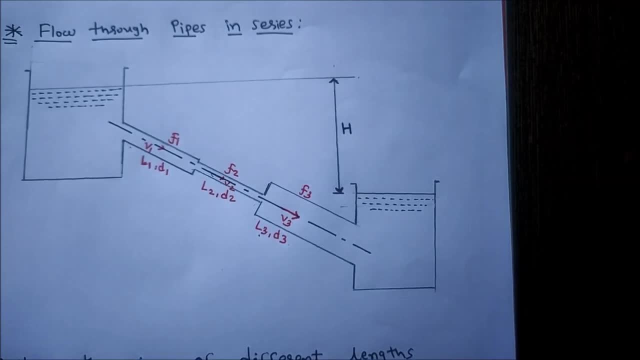 the pipes of different lengths and different diameters are connected end to end To form a pipeline, then such a pipe line is called as a compound or pipe in series, As the pipes are in series. that why the discharge through each pipe will be same. So according, 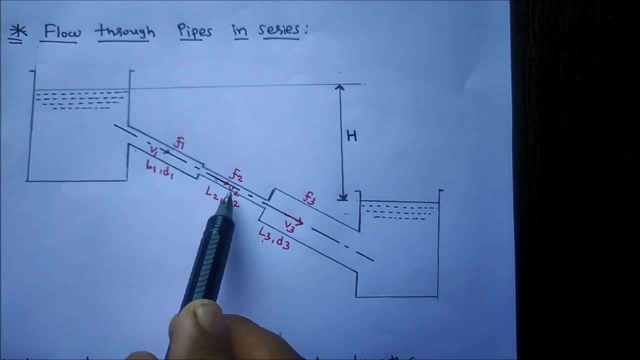 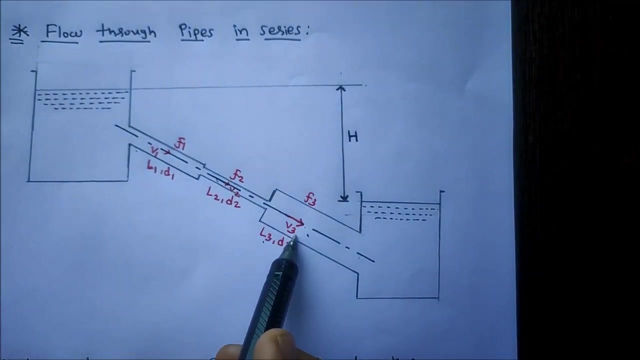 to continuity equation, Q is equal to A1, V1, equal to vice versa, Because here the pipes are in series. that's why discharge remain same. So, according to continuity equation, Q is equal to a1, v1 is equal to a2, v2 is equal to a3, v3 and the difference in 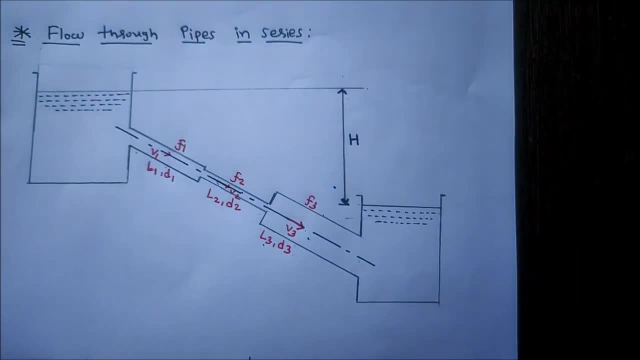 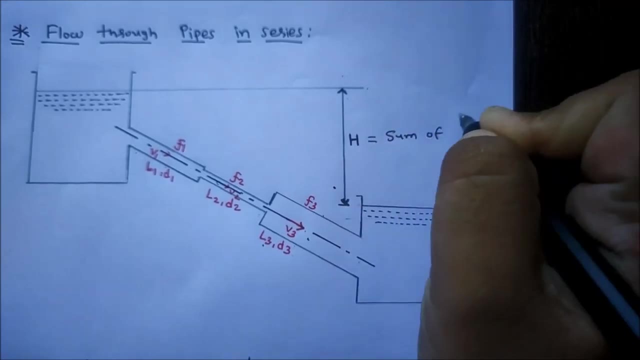 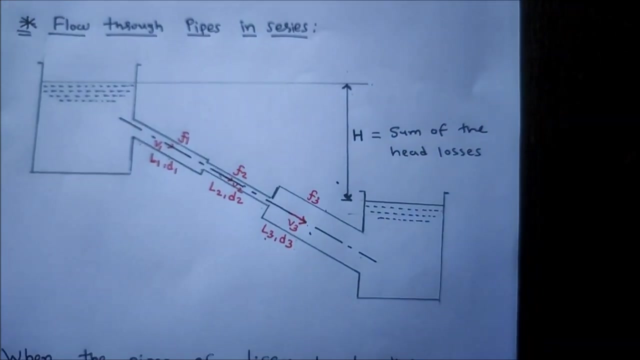 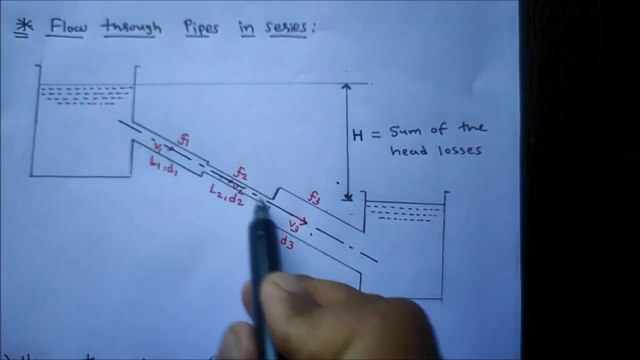 liquid surface level, that is, capital H, is equal to the sum of the head losses in all the section. is equal to the sum of the head losses in all the section. we know that when the fluid is flowing through the pipe, the fluid experiences some resistance, due to which some of the energy of the fluid is lost, so some of 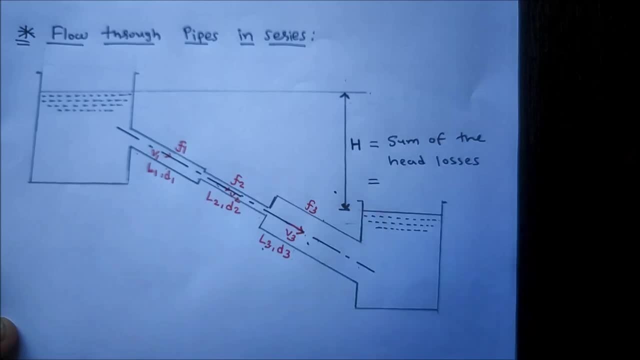 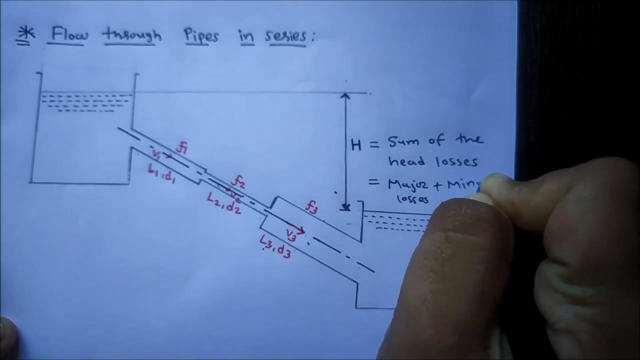 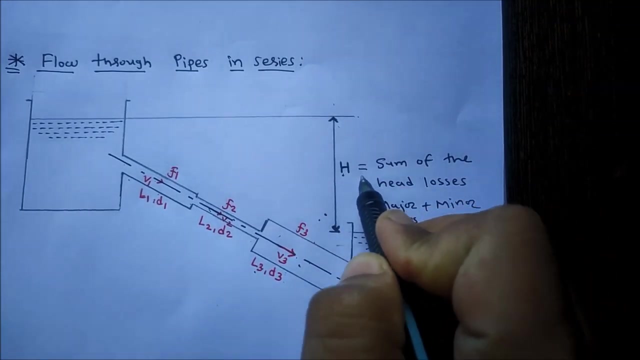 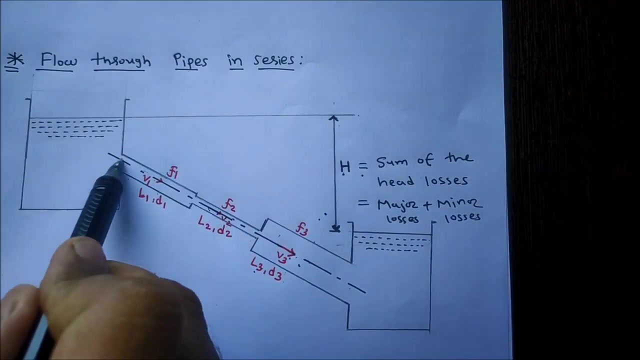 the head losses, that is the summation of major losses plus minor losses. so here the difference in liquid surface level, that is H. that is equal to the sum of the head losses in all the section. we know that when the fluid is flowing through the pipe the fluid experiences some 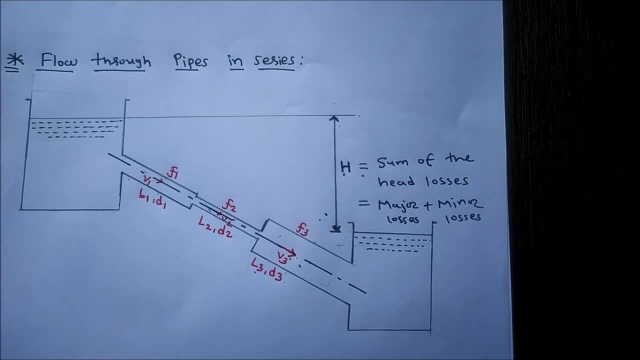 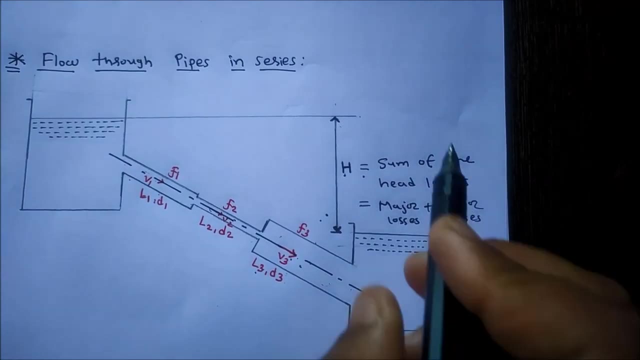 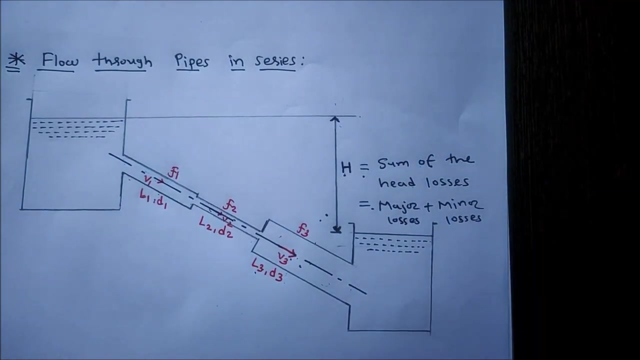 resistance, due to which some of the energy of fluid is lost. this loss of energy is classified as major losses plus minor losses, so some of the head losses, that is equal to the sum of the major losses plus some of the minor losses. so first we discuss about minor losses. 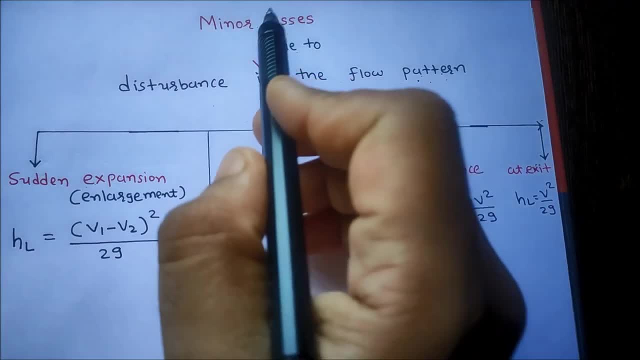 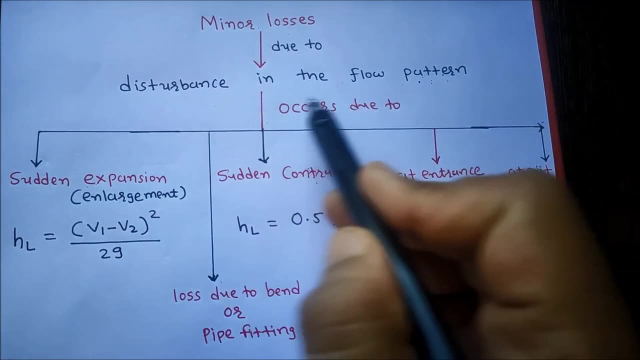 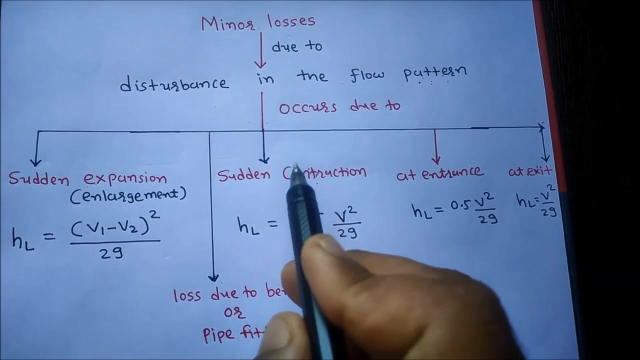 final losses. so what is the meaning of minor losses? minor losses means the losses due to the disturbance in the flow pattern. so when there is a disturbance in the flow pattern, this is in the flow pattern- happens when there is a sudden enlargement, there is a sudden contraction at entrance, at 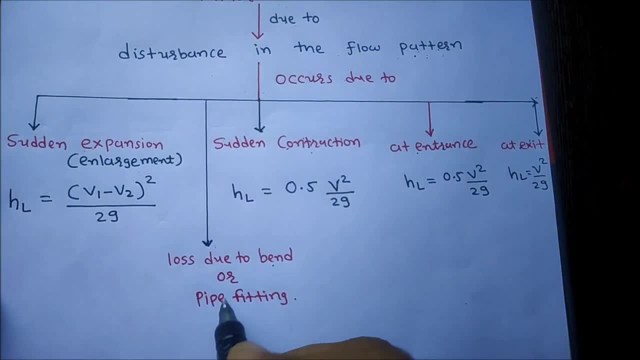 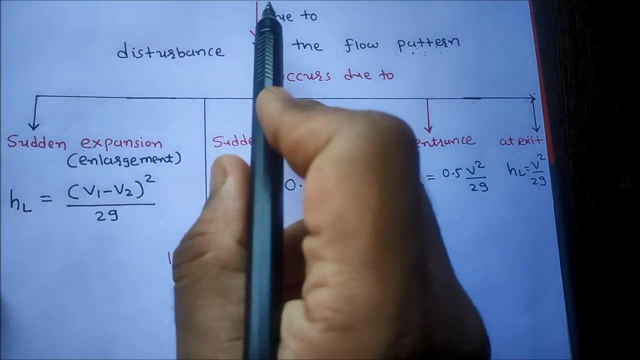 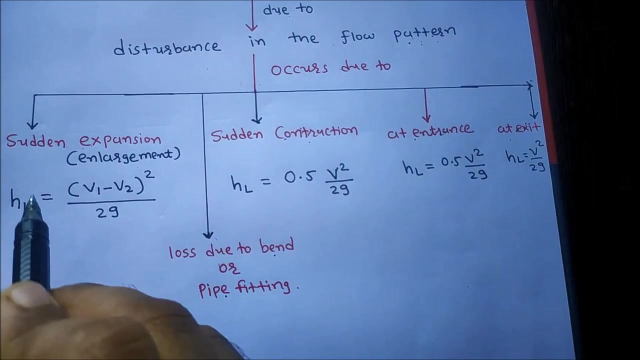 exit pipe is better by fittings. so that are the cases at where there is a disturbance in the. so minor losses happens when there is a sudden enlargement. so loss due to sudden enlargement- that's equation- is head loss. that is v1 minus v2, whole square divided by 2g. second one is loss due. 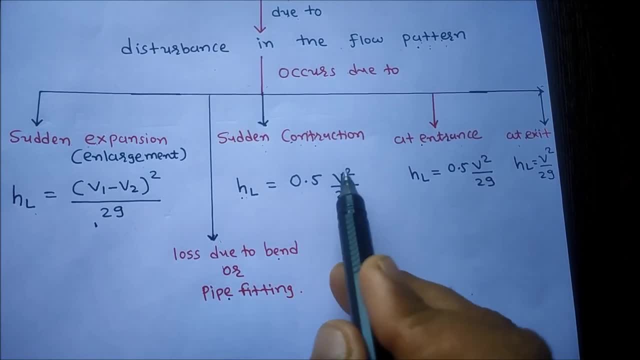 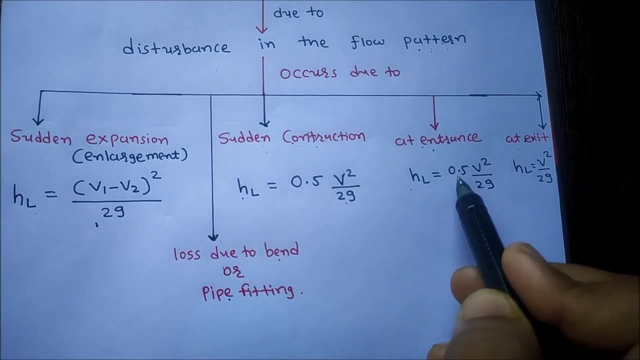 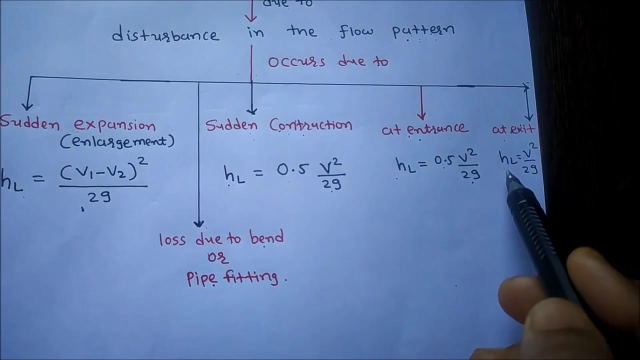 to sudden contraction means hl is equal to 0.5 v square by 2g. third loss, that is loss at the entrance. so head loss that is 0.5 v square by 2g. next is loss at exit from the pipe, so hl is equal. 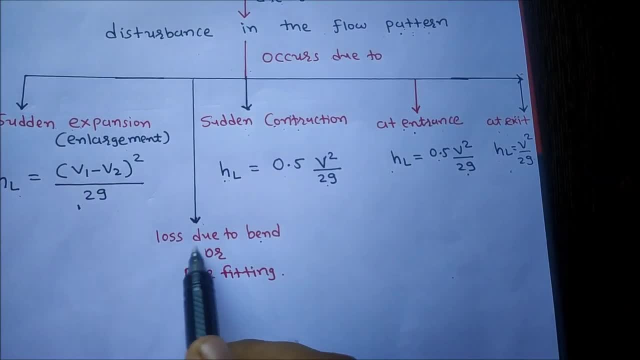 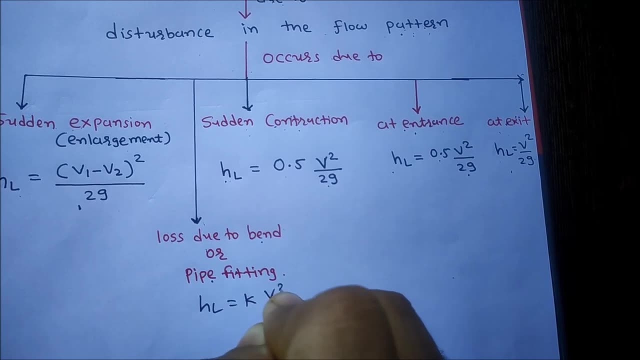 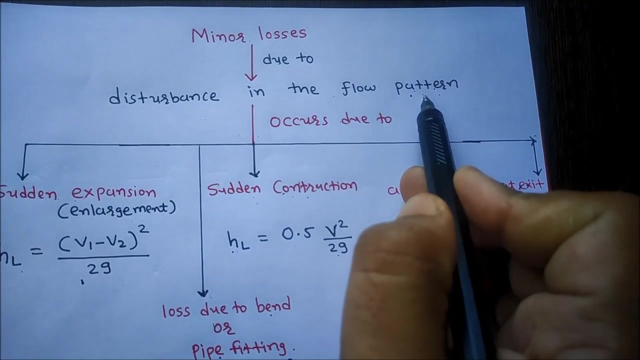 to v, square by 2g. and last one is loss due to bent or pipe fittings. that's equation is: hl is equal to k v square by 2g. so minor losses, that means the losses due to the disturbance in the flow pattern and when there is a disturbance in the flow. 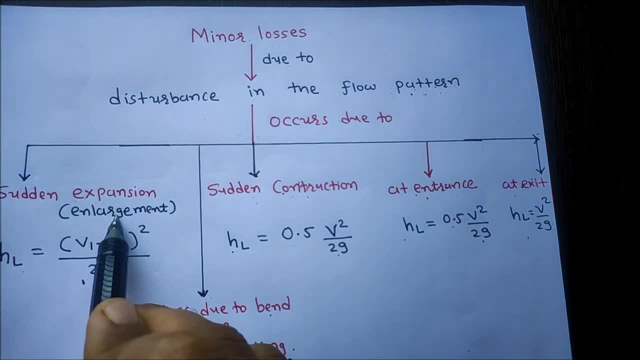 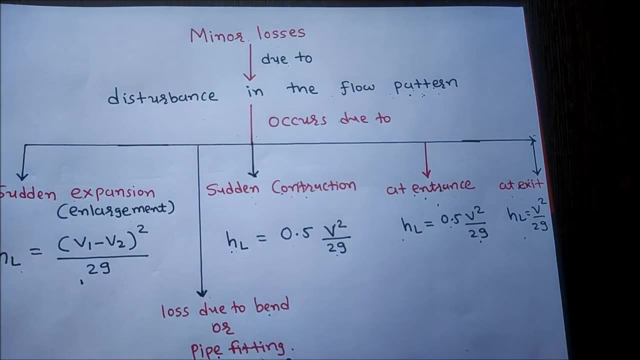 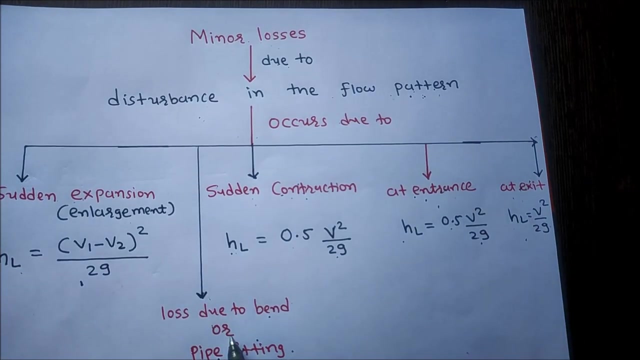 2g pattern. so disturbance of the flow pattern happens when there are sudden enlargement, sudden contraction at entrance, at exit bending or pipe fitting. so that are the cases at well there is a disturbance in the flow pattern. so these are responsible for minor losses. so we remember this equation. head loss due to sudden expansion, head loss due to sudden contraction at entrance. what is head loss at exist and head loss due to bend or pipe fittings. so in our case here the fluid enters the pipe, so there is a entrance loss that we already discussed. that equation is 0.5 and what is the? 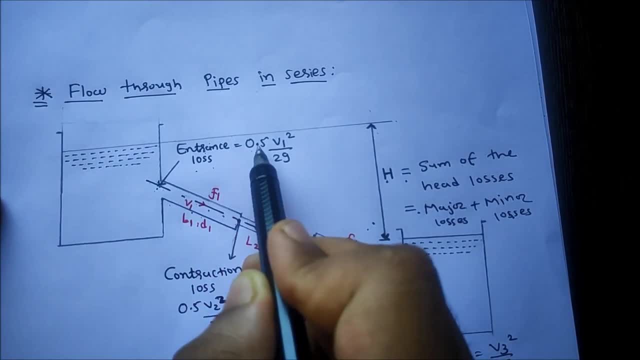 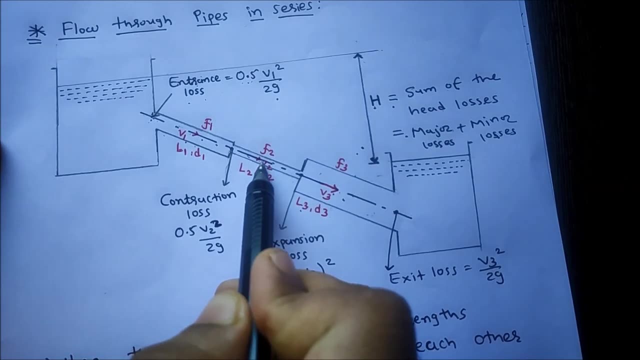 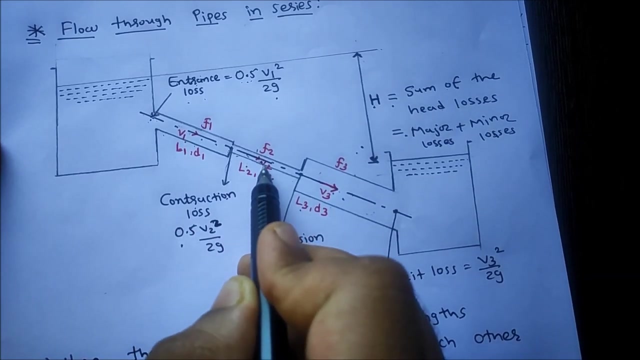 entrance, that is v1. so entrance loss is equal to 0.5 v1 square by 2 g. similarly, here diameter is decreasing, so there is a sudden contraction, so contraction loss: that is 0.5. here velocity is v2, so 0.5. 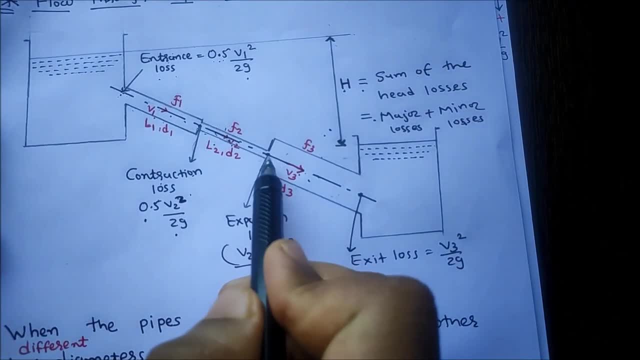 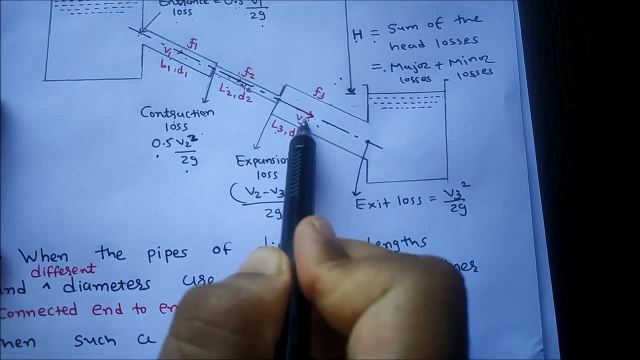 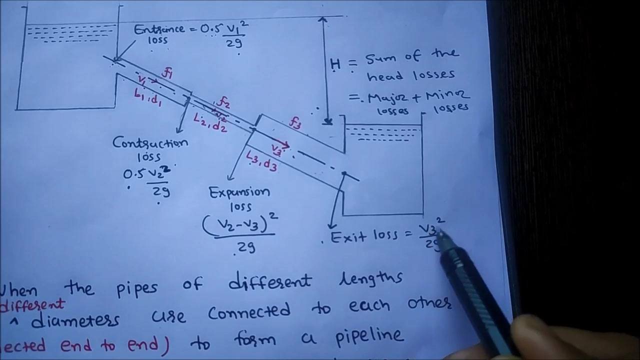 V2 square by2 g. similarly, there is sudden enlargement or sudden expansion, so expansion loss that we get here V2 minus V3, whole square divided by 2 g. and last one is fluid is exit. so exit loss that is v3 square by 2 g, because fluid exit velocity there is V3. 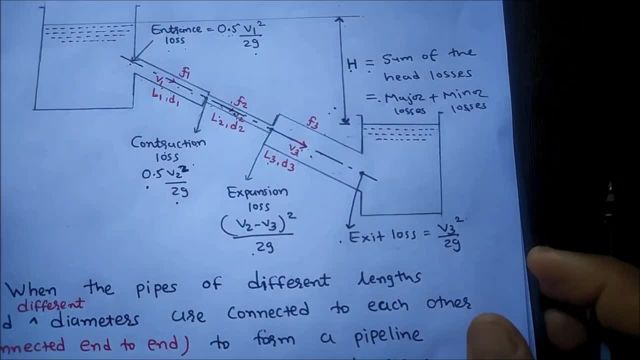 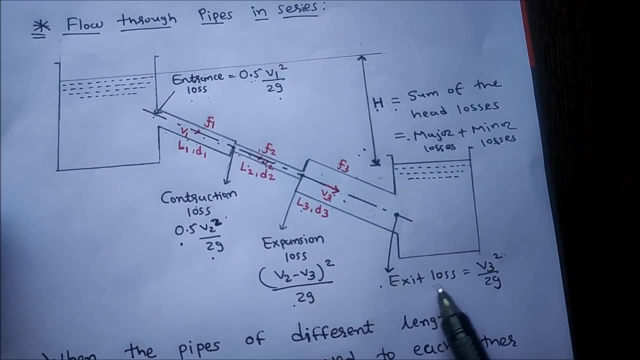 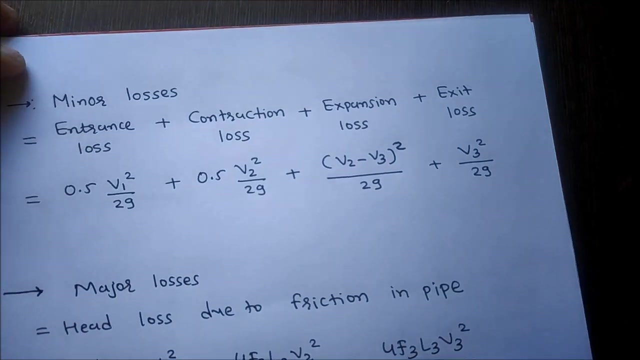 so exit is V3 square by 2G. So that are the minor losses: Entrance loss, contraction loss, expansion loss and exit loss. So first we write what are the minor losses. Minor losses is equal to entrance loss plus contraction loss, plus expansion loss plus exit loss and put the value of these losses. 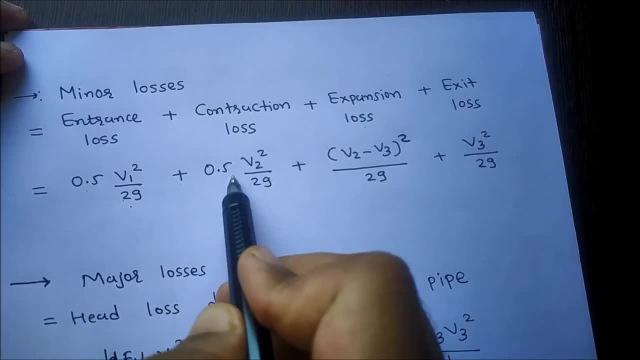 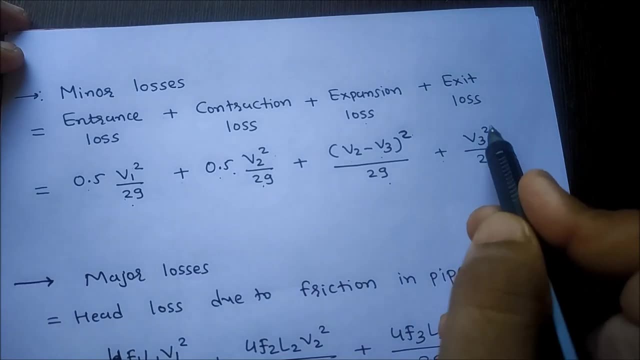 that is 0.5 V2 square by 2G. plus contraction loss, that is 0.5 V2 square by 2G. plus expansion loss, that is V2 minus V3 whole square by 2G, plus exit loss, that is V3 square by 2G. So what is the total? 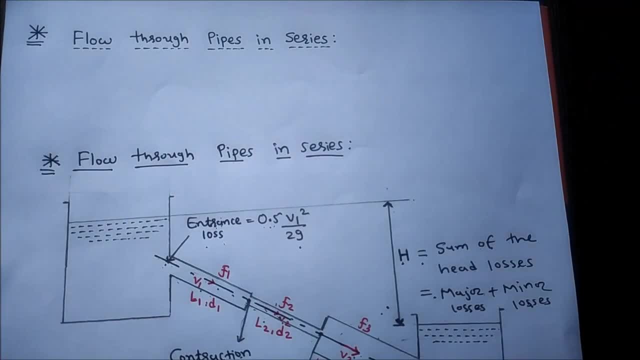 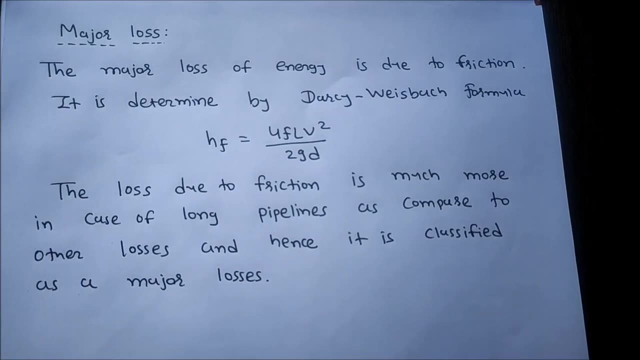 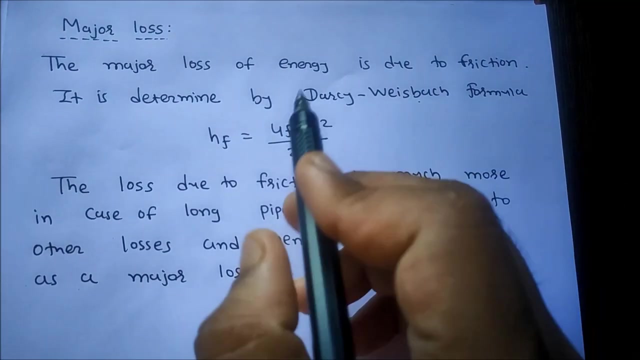 head loss. Head loss, that is the minor losses plus major losses. So H is equal to sum of the head losses, that is, major losses plus minor losses. So what is the meaning of major loss? The major loss of energy is due to friction and it is determined by Darcy-Weisbeck formula. and what? 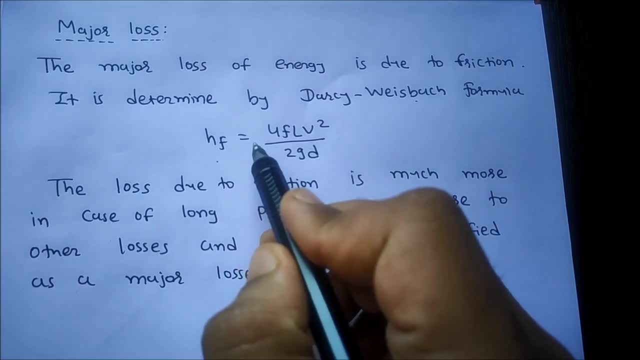 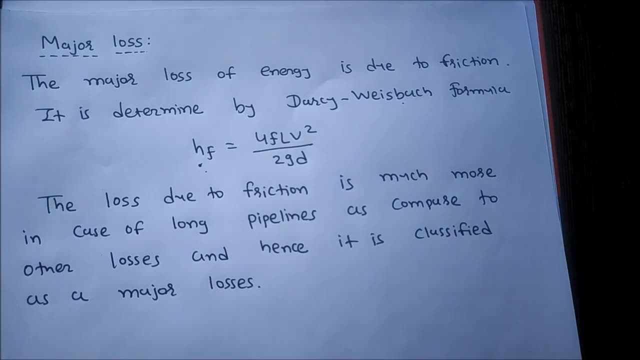 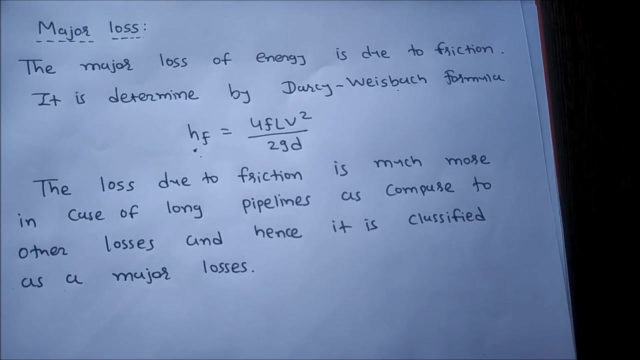 is the Darcy-Weisbeck formula, That is, HF is equal to 4F LV square divided by 2G, Where HF is equal to loss of head due to friction. So the loss due to friction is much more in case of a long pipelines as compared to other losses, and hence it is classified as major losses. 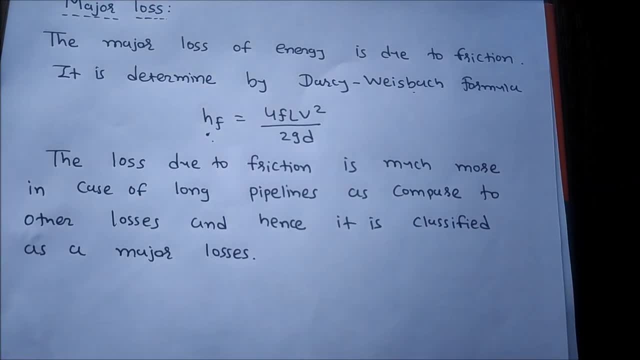 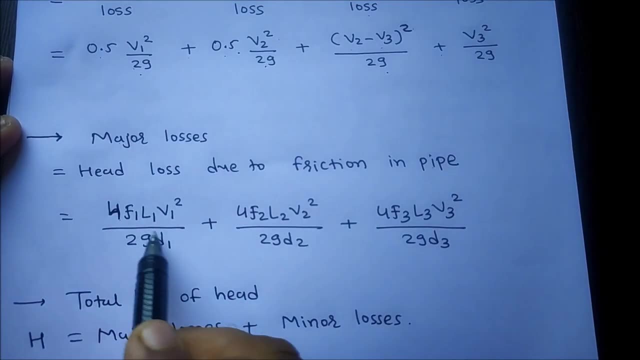 Now we calculate major losses. So head loss due to friction in pipe. So there are three pipes. So head loss due to friction in pipe that is 4F1- L1- V1 square by 2G D1, plus 4F2- L2- V2 square by 2G. 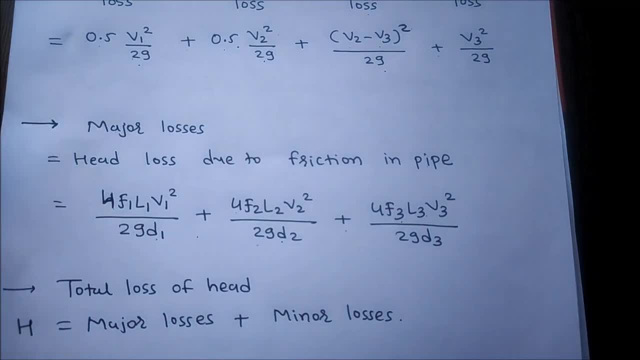 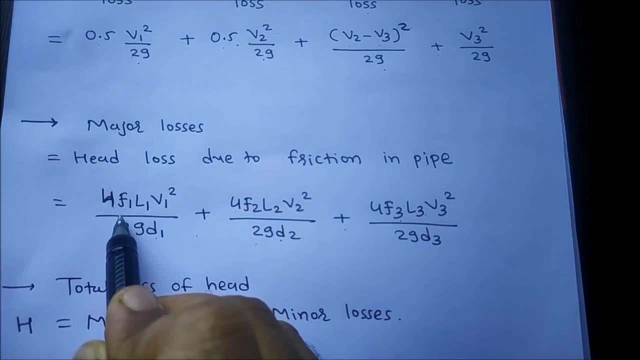 plus 4F3, L3, V3, square by 2G, D3. Here, F1, F2, F3, that is the coefficient for pipe 1, 2, 3.. L1, L2, L3, that is length of pipe 1, 2, 3 respectively, And D1, D2, D3, that is diameter of the pipe: 1, 2, 3 respectively. 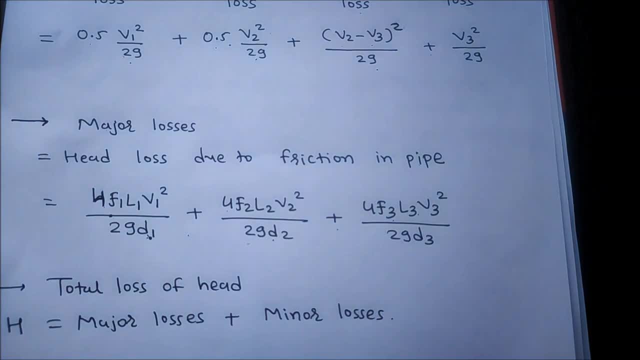 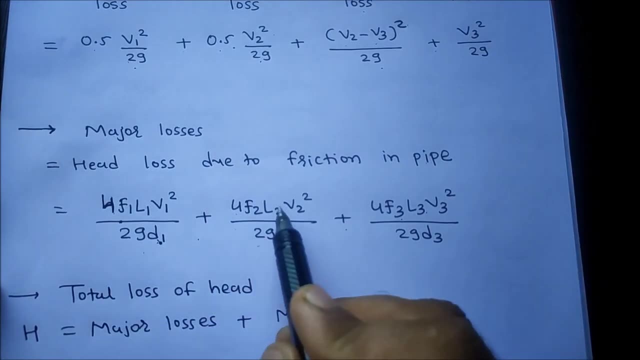 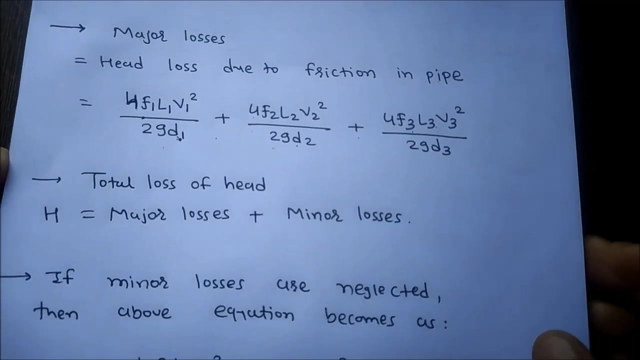 And V1, V2, V3, that is the velocity flow through pipes 1, 2, 3.. So major losses equation: that is the 4F1L1 V1 x 2G D1.. F2- L2, V2 square by 2G D2, plus 4 F3, L3, V3 square by 2G D3.. So total loss of head, that is h is. equal to major losses plus minor losses, Simply put, the value of minor losses and major losses. So in case of short pipe minor losses is to be considered, whereas in long pipe it does not make any serious effect. That's why, if minor losses are neglected, then above equation becomes as: 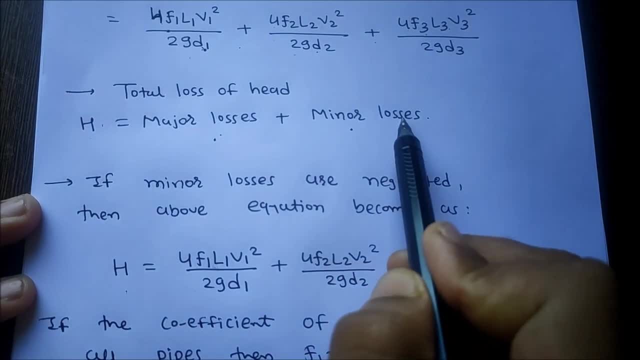 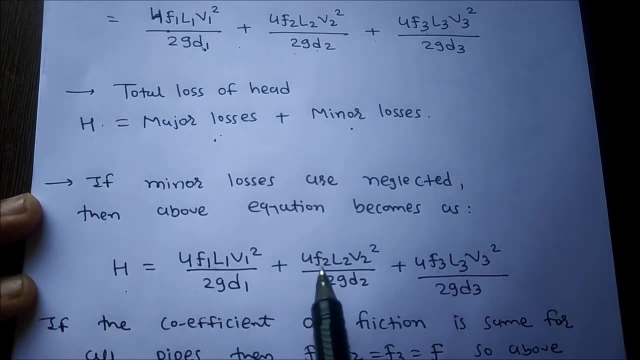 capital H is equal to minor losses. neglected that means capital H is equal to major losses and major losses equation: that is 4 F1 L1 V1 square by 2G D1, plus 4 F2 L2- V2 square by 2G D2. 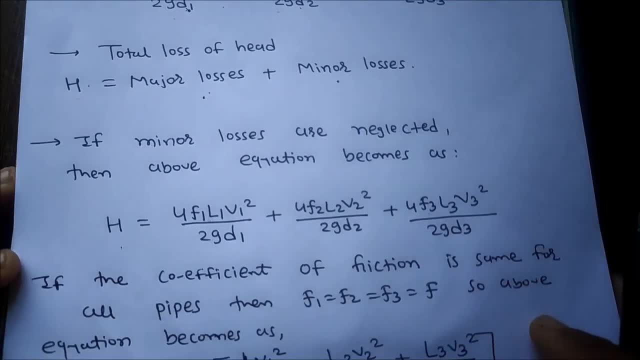 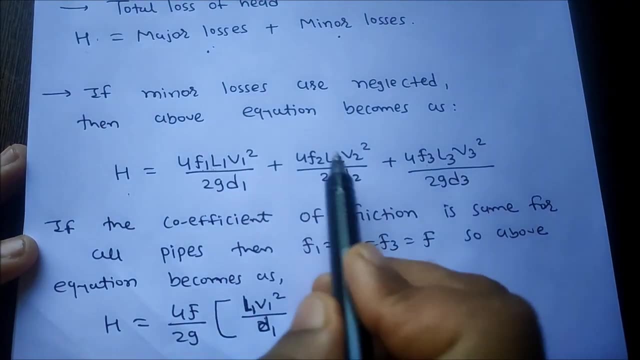 plus 4 F3, L3, V3, square by 2G, D3.. So if the coefficient of friction is same, that is, F1 is equal to F2 is equal to F3. So above equation becomes as: 4 F by 2G, that is common. So H is equal to 4 F by 2G in. 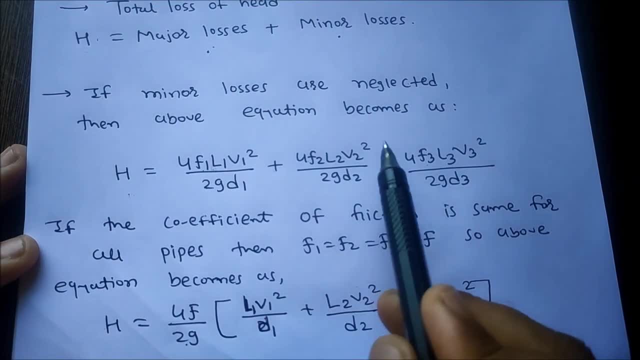 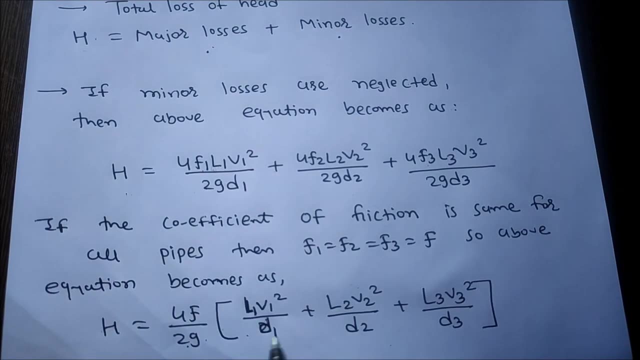 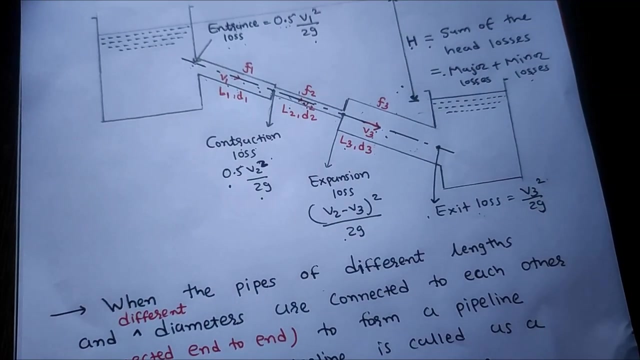 bracket: L1- V1, square divided by D1, plus L2. V2 square divided by D2, plus L3. V3 square divided by D3.. So that is the equation for flow through pipes in series or flow through compound pipes. Again, I repeat, Flow through pipes in series means what happens. So first of all, we have 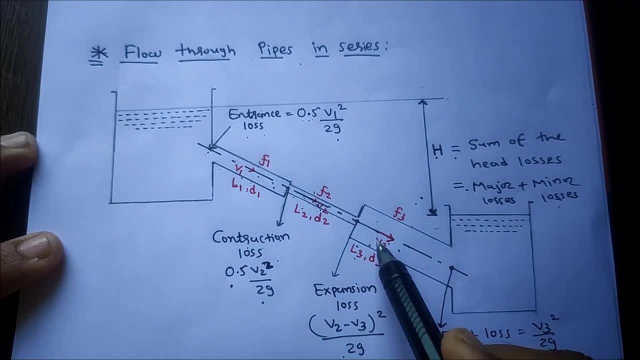 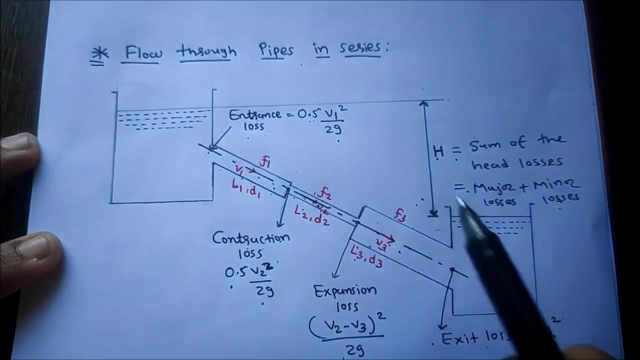 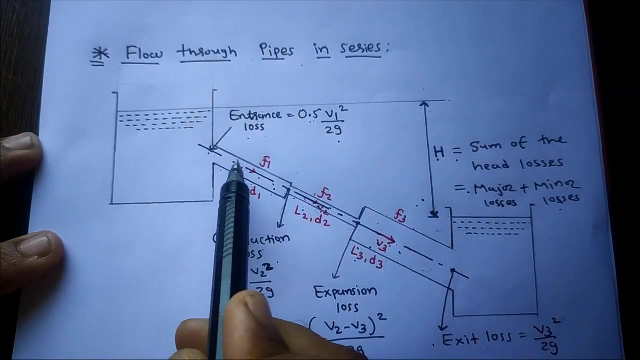 to consider 3 pipes. The length and diameters of 3 pipes are different. So if we connect the pipe of different length and diameters end to end, that means a pipe line will be formed. So we will call it pipes in series or compound pipes. Now, here pipe is in series. that means the rate of flow in. 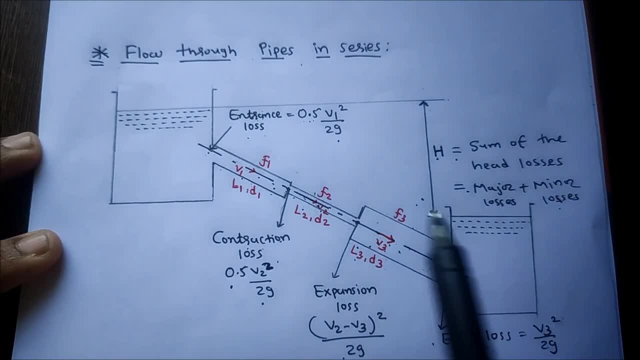 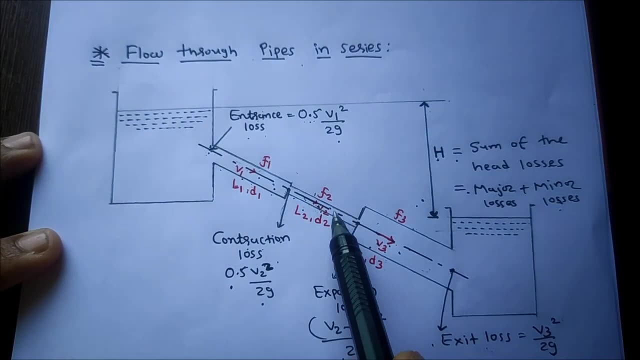 first pipe will be same as in second pipe and same as in third pipe. That means discharge will be same in all 3 pipes. So according to continuity equation, Q is equal to E1, V1 is equal to E3, V2 equal to A1, A1 is equal to A2, V2 is equal to A3- V3. 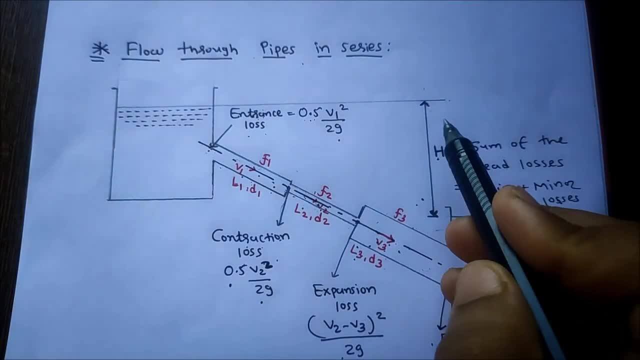 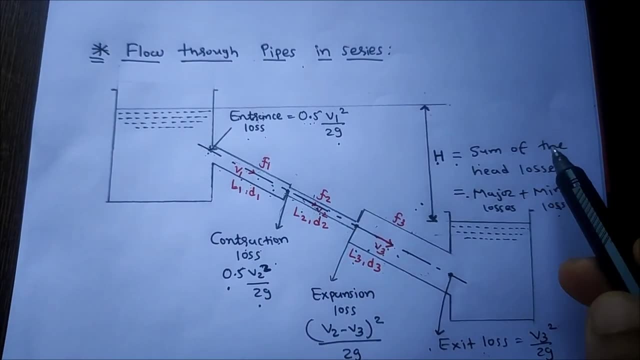 The difference in liquid surface level, that is H, is equal to total headлось in pipe. total headloss in pipe, that is the total headloss plus the total headloss inAC2, is equal to the total headloss in water pipe. So how will be total headloss 5 times? well, the total headloss. 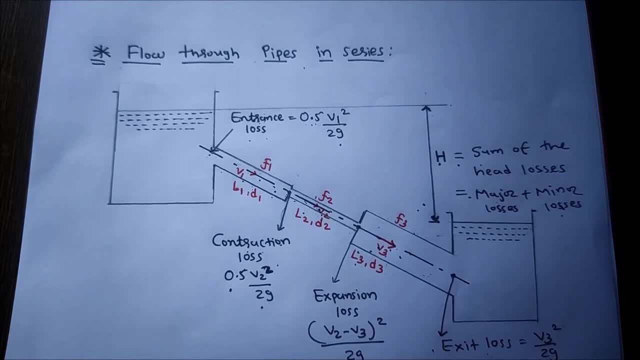 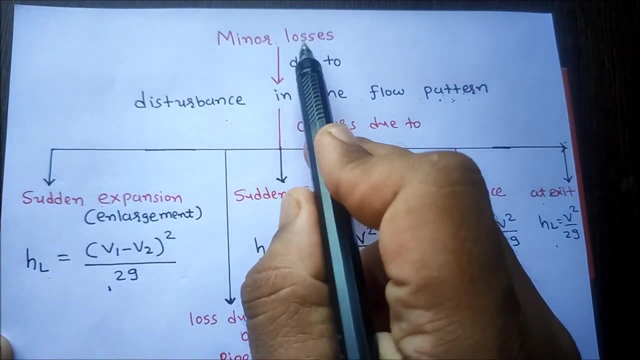 in water pipe. So we are going to discuss. gefragt about minor loss in water pipe. Now, what is the minor loss? Miner drop difference is defined as the loss of lipstick due to disturbance in the flow pattern. So the minor drop in water pipe is 0 because the loss is likely to increase or decrease. 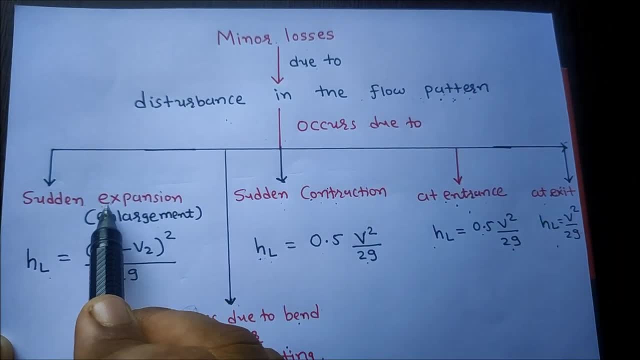 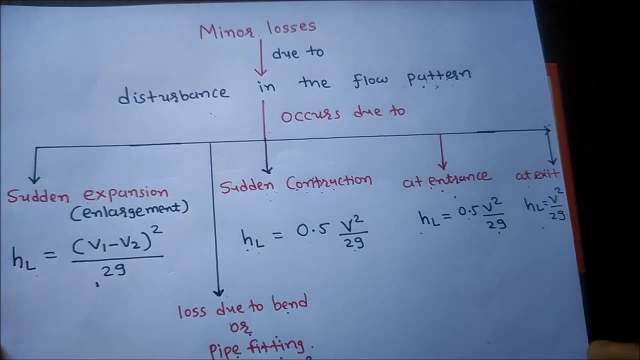 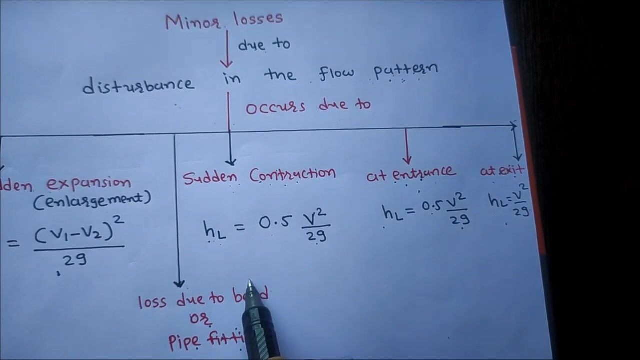 in the flow when there will be disturbance in flow pattern. there will be sudden expansion. if diameter is increasing suddenly, if diameter is decreasing suddenly, if there is sudden contraction at entrance, flow pattern will change. at exit it will change. if it is bending, that means there will be disturbance. 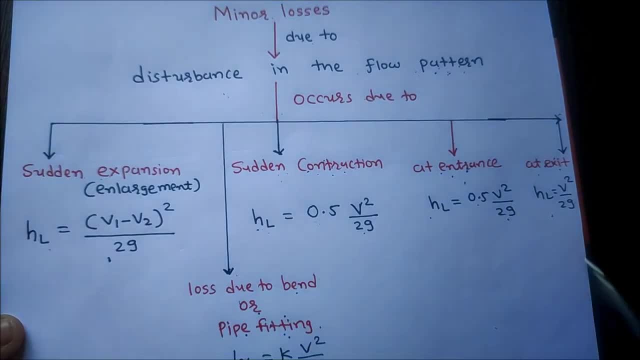 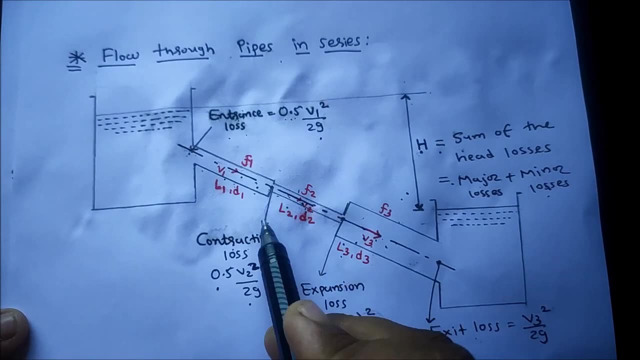 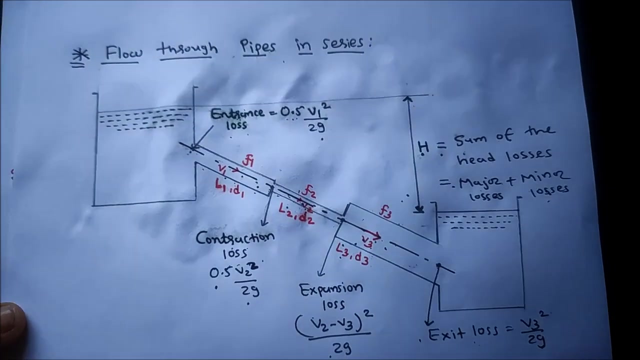 in flow pattern and pipe fitting. so we have to remember all these equations. and in our case, here fluid is entering, that means entrance flows. there is a sudden contraction. suddenly diameter is decreasing, that means contraction loss. here diameter is increasing, that means expansion loss. here fluid is exiting, that means exit loss. 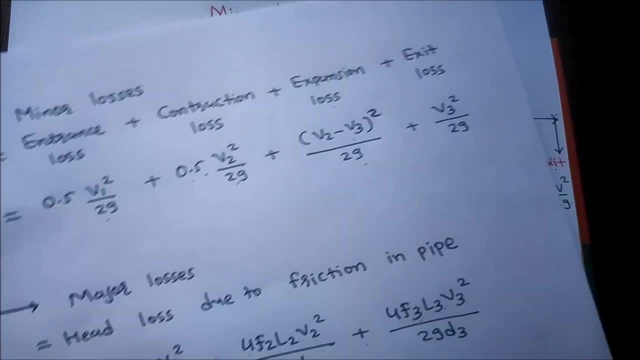 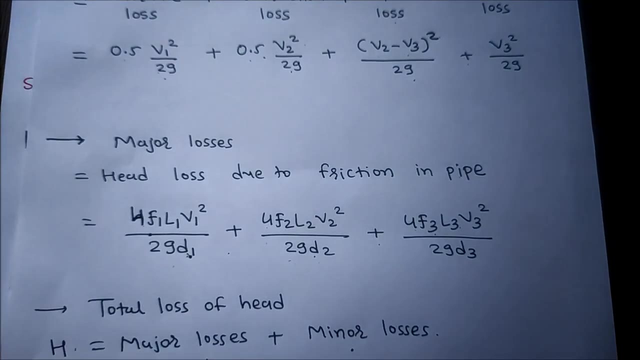 so if we will do all these summation, then we will get minor losses, so we got equation of minor losses. similarly, we will find equation for major losses. so in major loss which equation is used? that is Darcy-Weisbach equation. so for all three pipes. 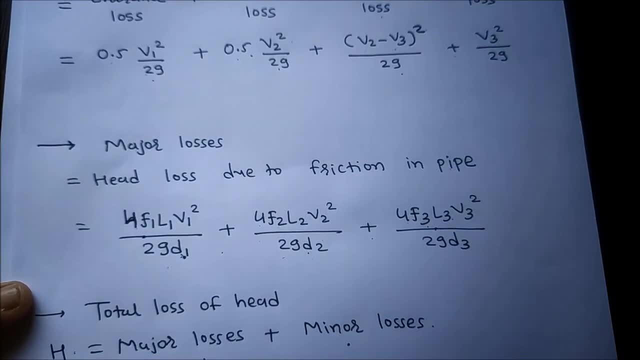 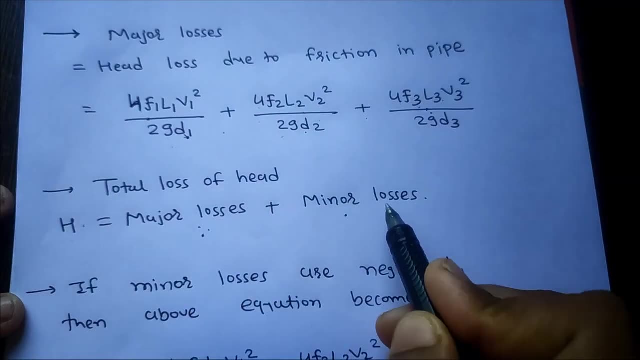 we will use Darcy-Weisbach equation. so what is major losses? and we use Darcy-Weisbach equation, so what is total loss of head capital H is equal to major losses plus minor losses. here we will keep value in equation, so we will get total loss of head. 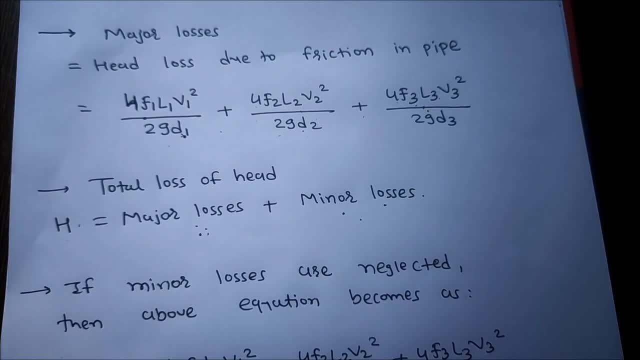 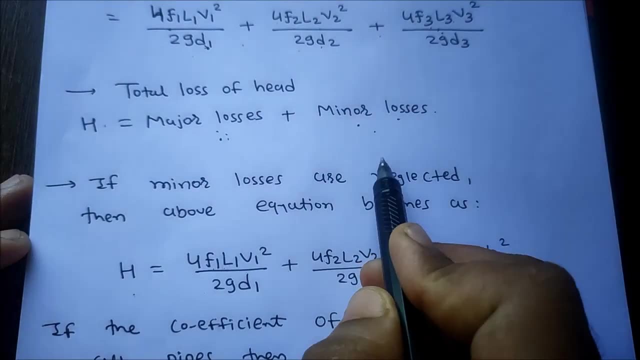 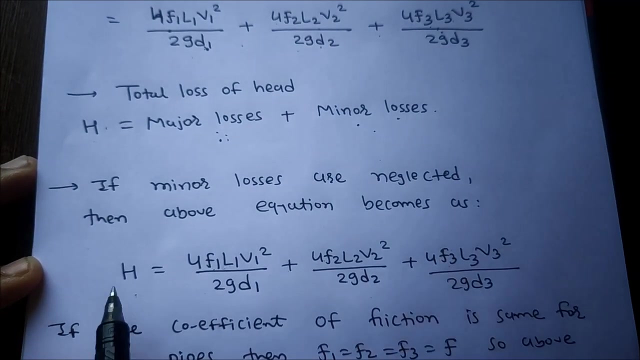 but if pipe is short, then we will consider minor losses. but when pipe is long that means it does not make any serious effect. so here minor losses we will neglect. so what is total loss? of head H is equal to major losses. so here again we will keep equation of major losses. 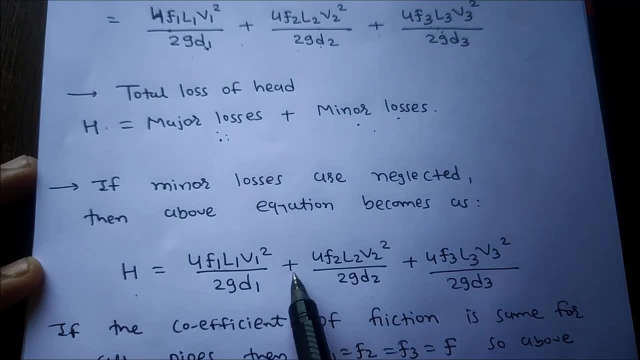 capital H is equal to 4F1L1V1 square by 2G D1 plus 4F2L2V2 square by 2G D2 plus 4F3L3V3 square by 2G D3. 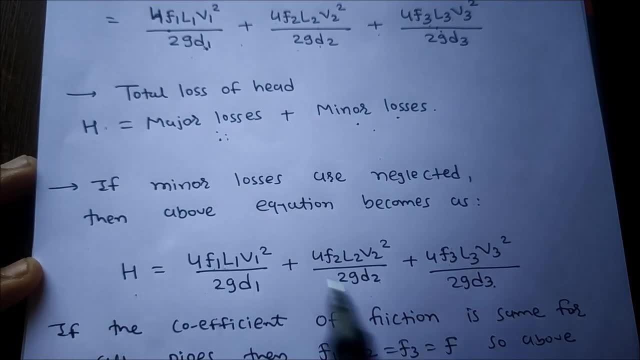 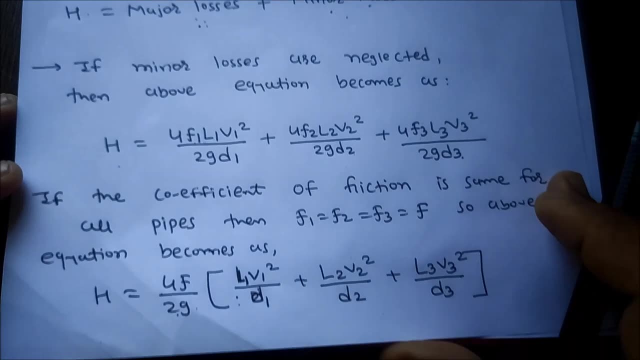 but here coefficient of friction for all pipes. if same, that means F1 is equal to F2 is equal to F3, so we will get 4F by 2G common. so capital H is equal to 4F by 2G in bracket.